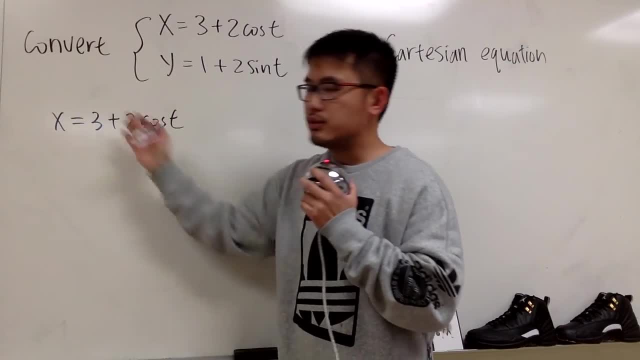 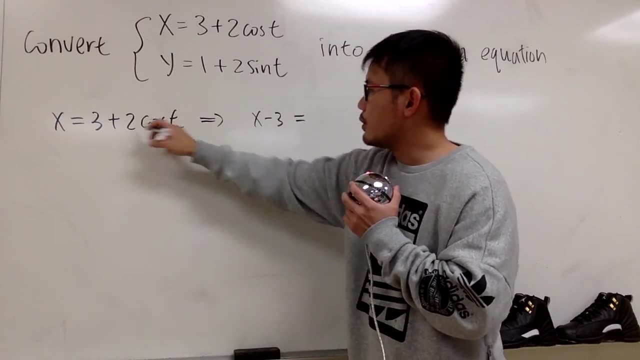 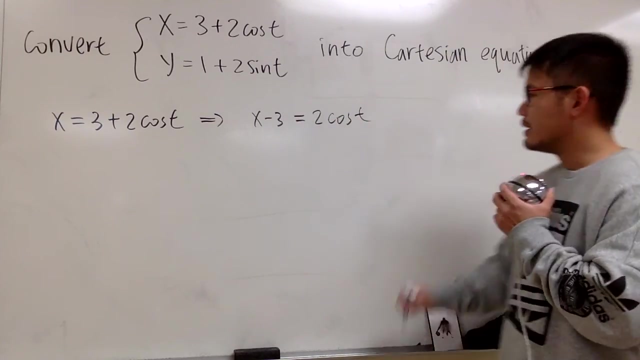 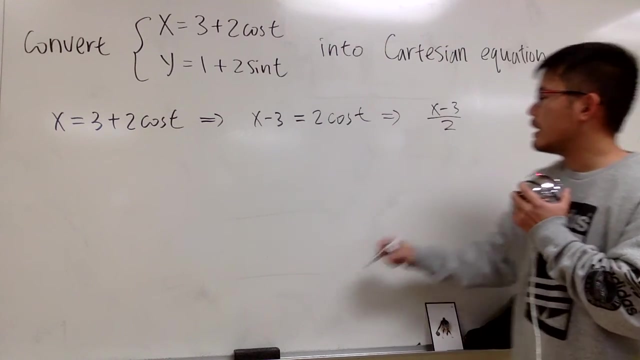 and then do the usual deal, That's minus 3 on both sides. This is going to give us x minus 3 equals to 2 cosine t, and then we can definitely divide both sides by 2.. So at the end we have x minus 3 over 2, equals to cosine t, right? 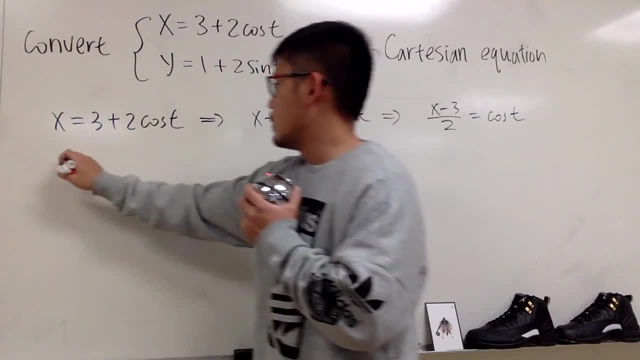 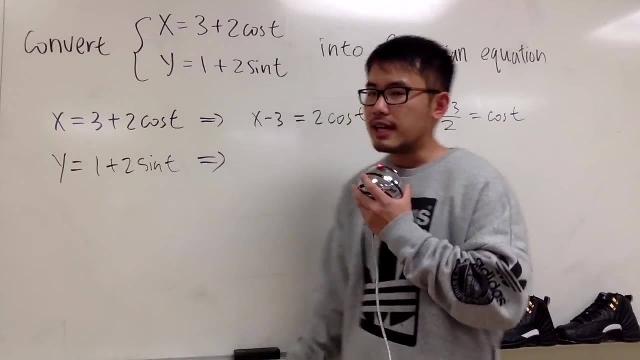 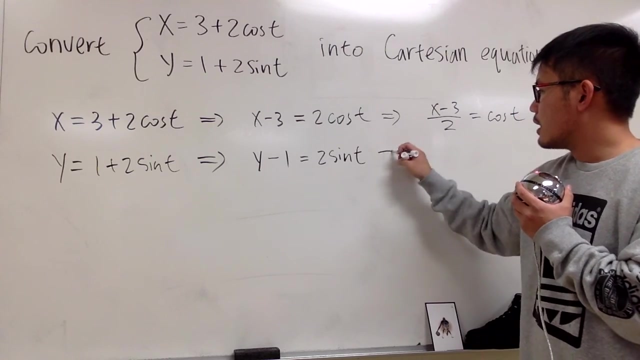 And we will do the similar things With the y equation. y is equal to 1 plus 2 sine t, and this is going to give us minus 1 on both sides. So we have y minus 1, and that will give us 2 sine t and then divide both sides by 2.. 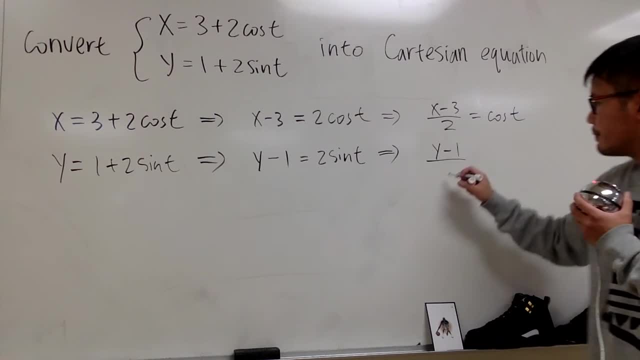 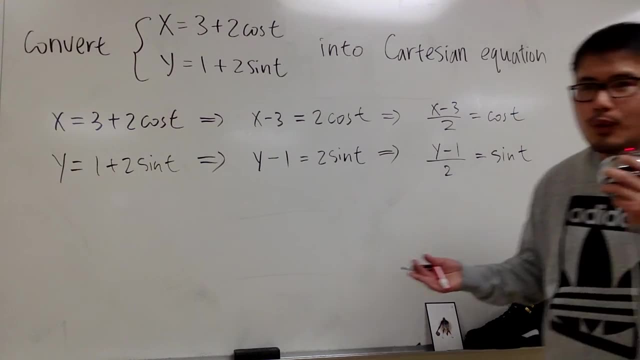 So we have y minus 1 over 2, and that will give us sine t. And you may be wondering: what good does this do? Well, the deal is that when you have cosine and sine, if the angles inside are the same, 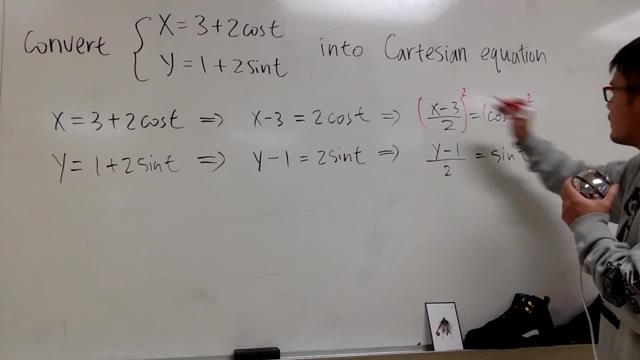 we can just square both sides. So this is the first one that we have, and likewise, we'll do the same thing right here as well. At the end, this is going to give us what? Look at this: We have x minus 3 squared. 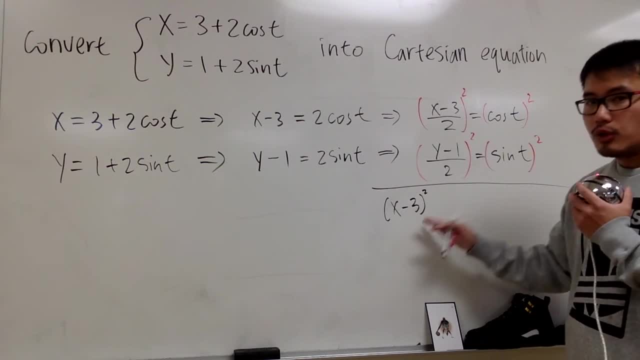 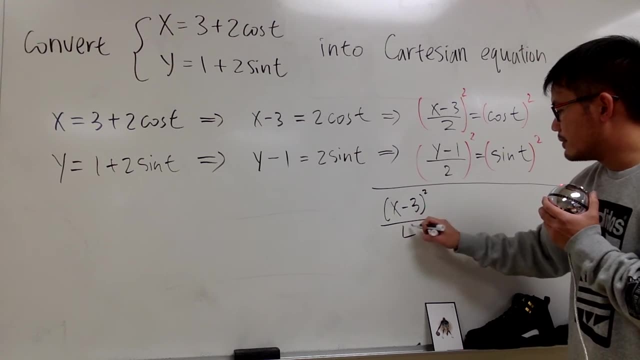 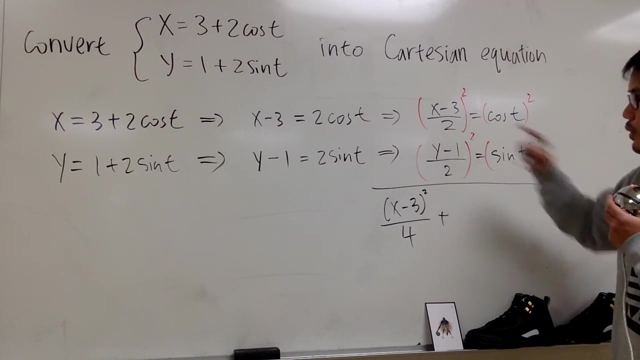 Let me put it down this way for you guys: x minus 3 squared, don't multiply this out. Let me put this down in parentheses like this: Over 2 squared, so we have this over 4, right? And then plus. we're adding these two equations together, so you're adding this quantity right here as well. 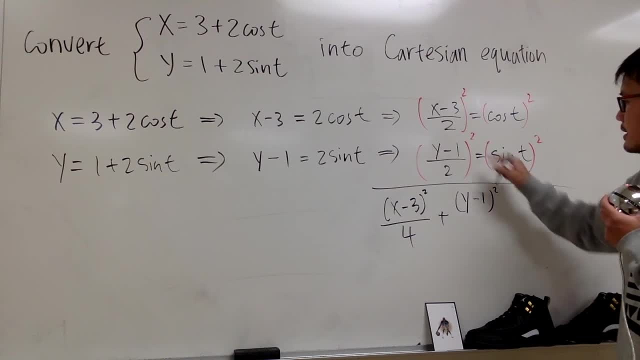 You have y minus 1 squared and then over 2 squared, and once again, I'm keeping the top and I'm squaring the bottom like this At the end, if I add these two equations, what do we get? 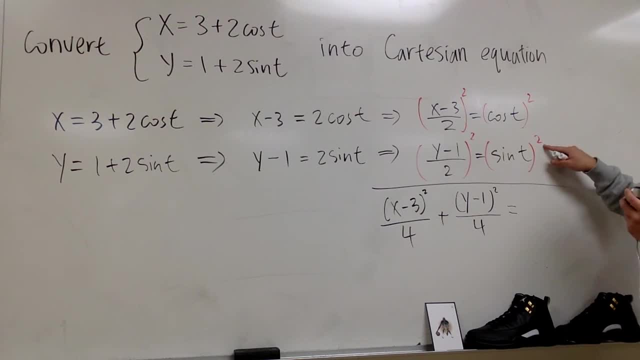 What do we get? Cosine squared plus sine squared will be equal to 1, when the angles that we have, it's the same. So we have this and this is equal to 1, right? So this is pretty much it.